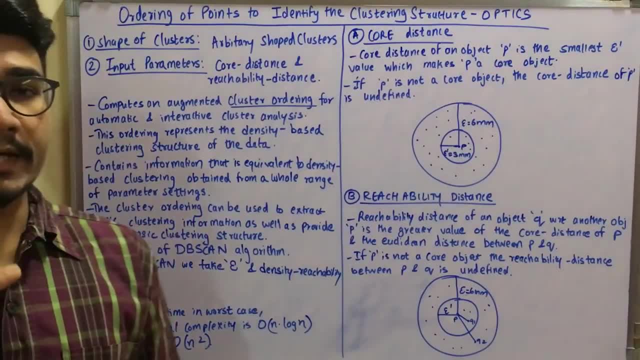 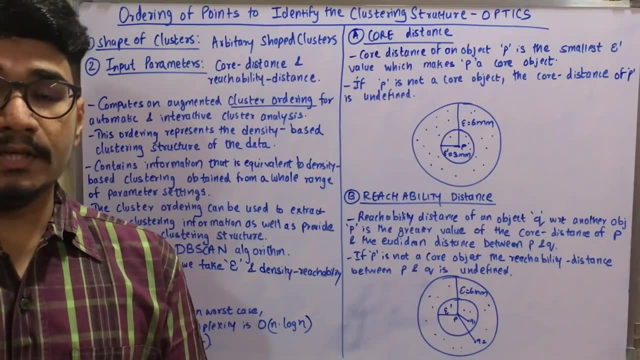 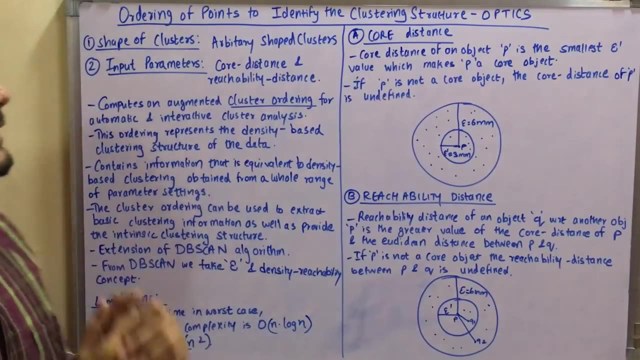 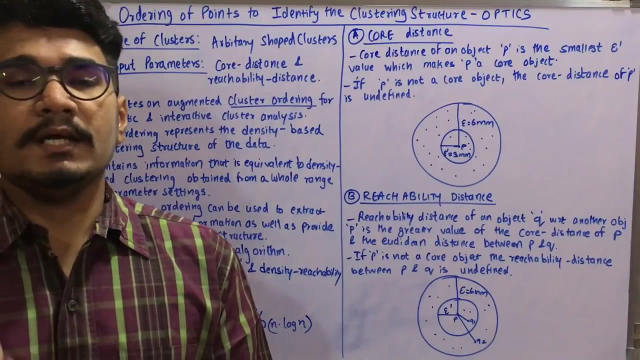 noise and all So in this, what we have, we have the ordering of points. So some kind of cluster ordering or some kind of concepts are there So that we use to identify the clustering structure and also the intrinsic feature or other informations which are there in the cluster. So let's start. what is optics in data mining? So we have from the db scan what the downfall of db scan is that we have some parameters. we have epsilon, minimum points and also the core distance, And so 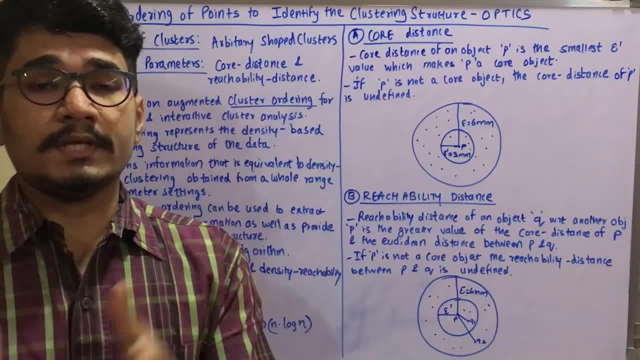 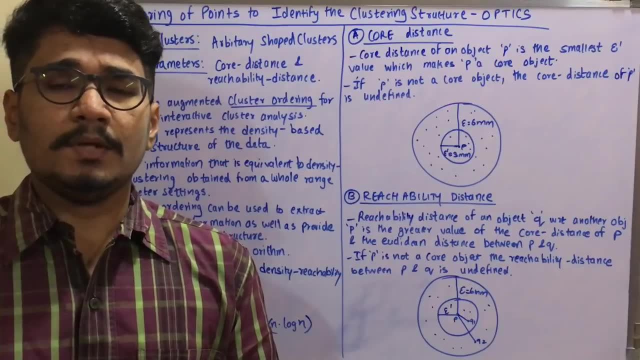 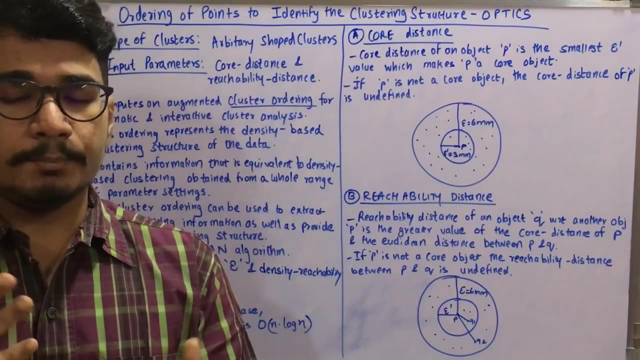 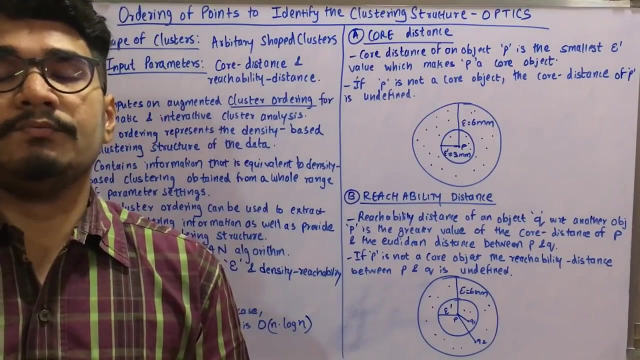 it's mainly concentrated on calculating or to segregating out the high density region. So it's like if any small slight variation in the decimal point or any slight shift in the values just here or in the left or right, then it may cause the distortion of that particular cluster or it may not properly identify that particular kind of cluster. So that was the very downfall of db scan And so it has to be very specific and very precise in terms of points. 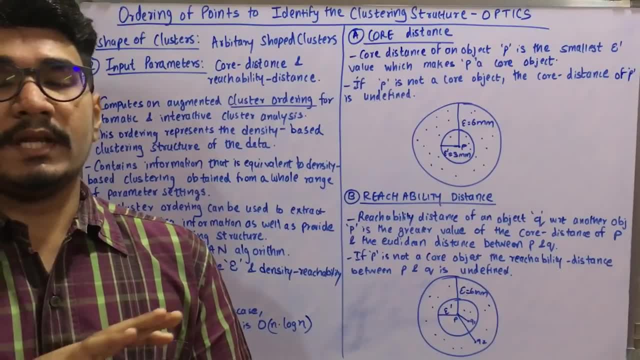 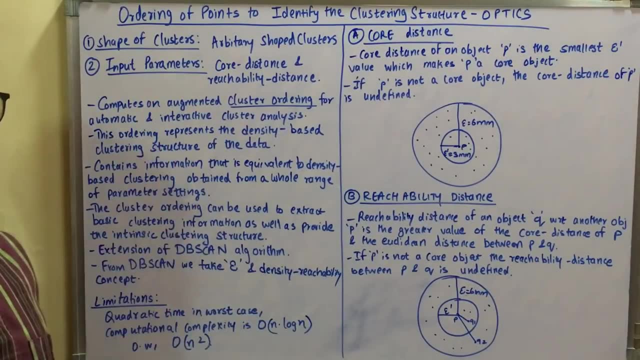 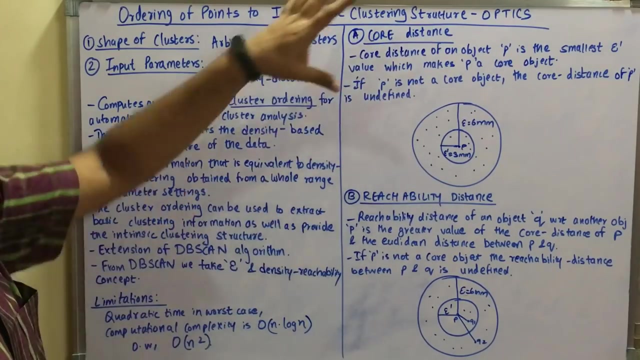 to identify it. So optics doesn't consider that thing. So it's like in a fashion of points you need to have in optics. So we start with the basic two parameters, that is, we have the shape of the cluster. So, since it is, a density based method is used for identifying the arbitrary shape clusters, and also the input parameters that it would be requiring is the core distance and the reachability distance. or main topic or main idea of optics would be on these two, that is, core distance and reachability distance. We'll see. what is it So before. 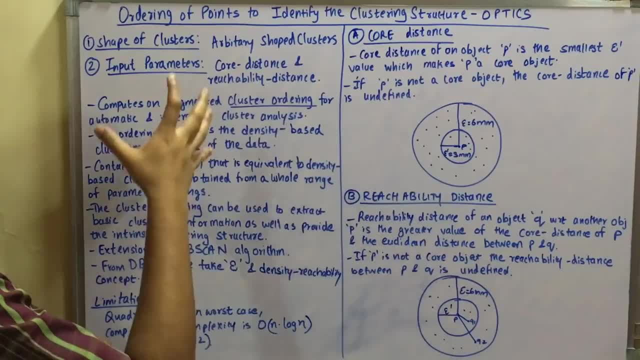 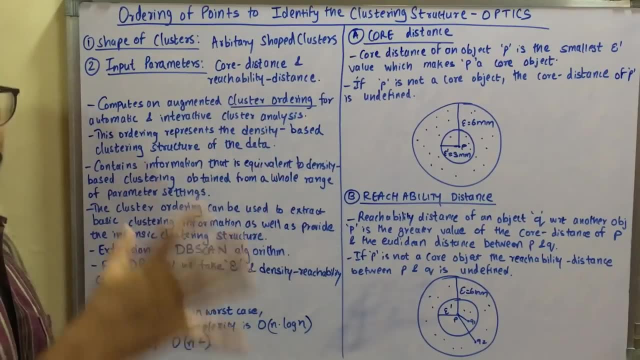 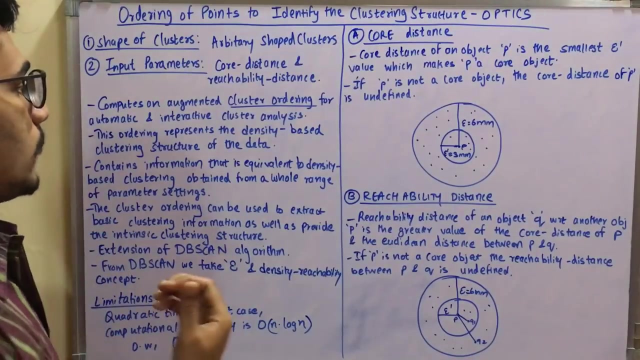 that we compute an augmented clustering order for automatic and interactive cluster analysis. So it's like an added benefit or added feature. which we have in optics is cluster ordering, So some kind of ordering might be there in the cluster to identify the data points or how it's laid out. So that's basically automatic. or it can be other interactive from the user perspective. it may be asking what points you have to enter and solve those kinds of information. So this ordering represents a density based clustering of the structure, So like. 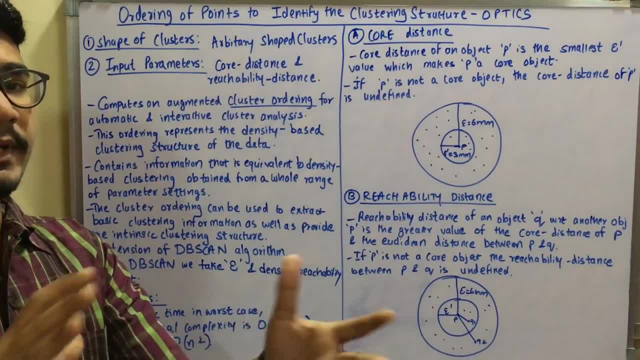 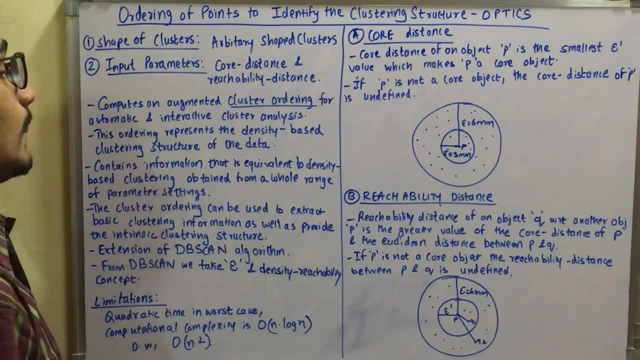 since it's like cluster ordering is there so we need to have the density based structure, or so it's like it falls in that category of density based methods. Then it contains information that is equivalent to density based clustering, obtained from a whole range of parameter settings. So it's like you have those density based clustering ordering for different clusters, And so it will be kind of different kinds of intrinsic information. the clusters shape the dimensionality and all those kinds of things. So the cluster ordering can be used to extract basic 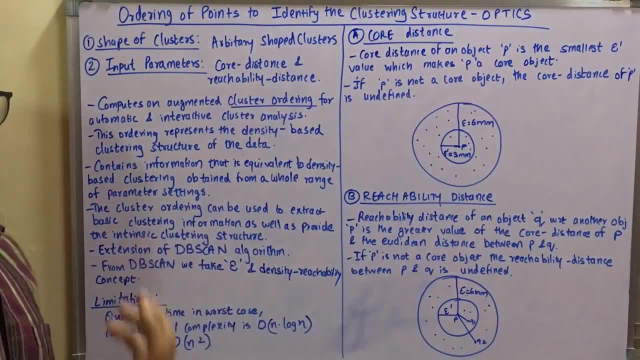 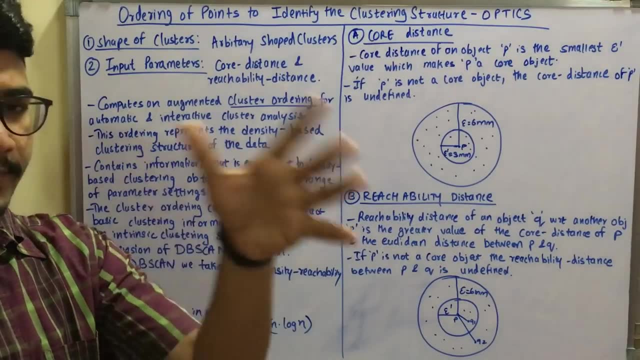 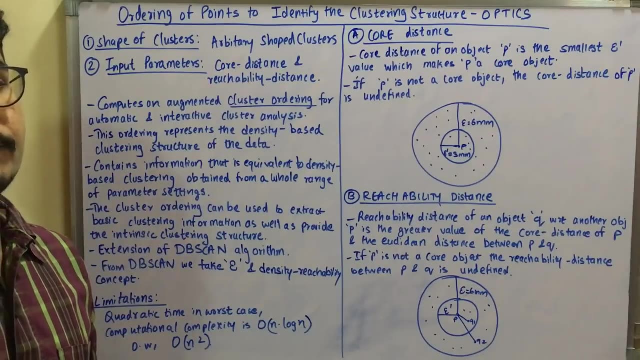 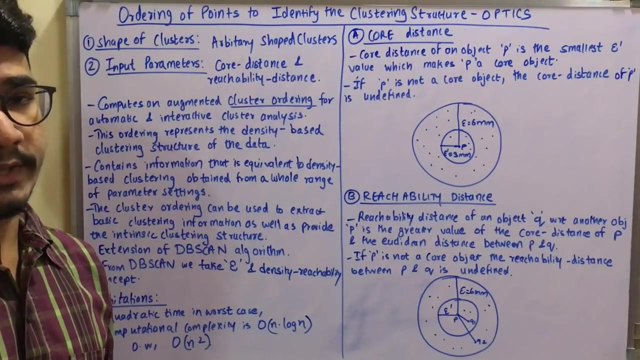 clustering information as well, as it can provide the intrinsic clustering structure, So how the different points are laid out, or what are the noise points, or what are the water points and how it's distance basically. So all these things gives you in optics, And so you can see that next reason of DB scan algorithm, which we have previously learned, and so if I'm seeing it's an extension of DB scan- some properties or some parameters it has to extract from DB scan, And so from DB scan we take the epsilon. that is the minimum distance. 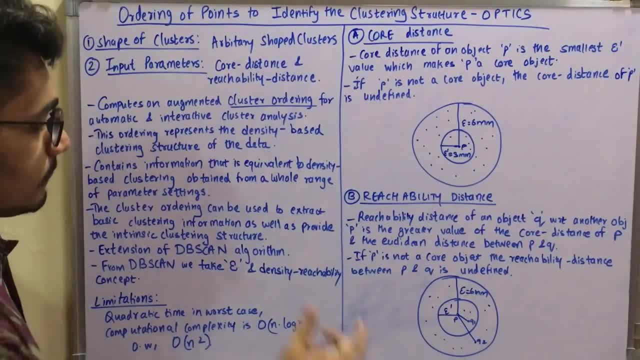 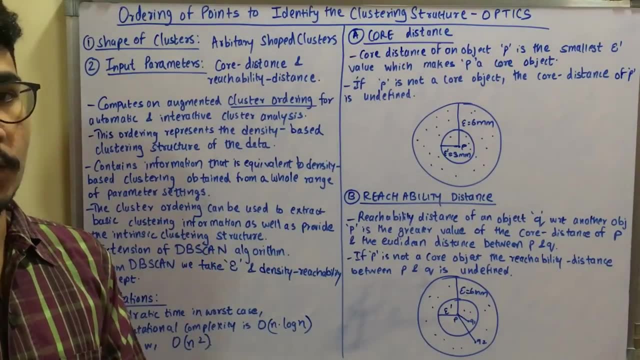 of the cluster of the core point to reach the other points or the noise points. and then you have the density reachability concept. so these two concepts will just take to in order to drive or to design the optics clustering technique, and so we'll move on to the limitation last. so limitation is nothing. 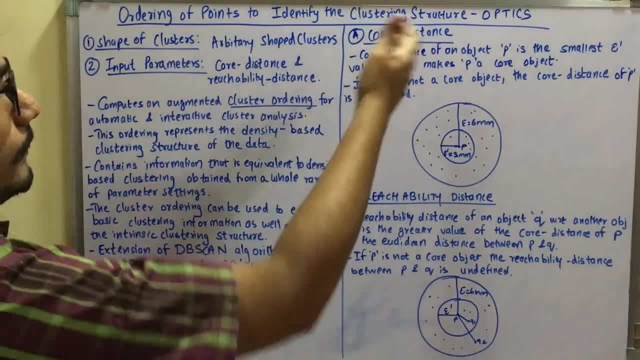 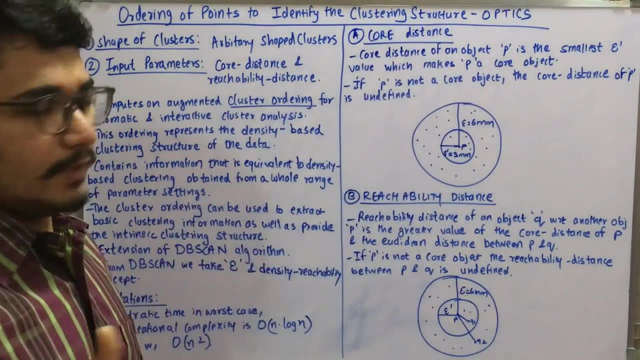 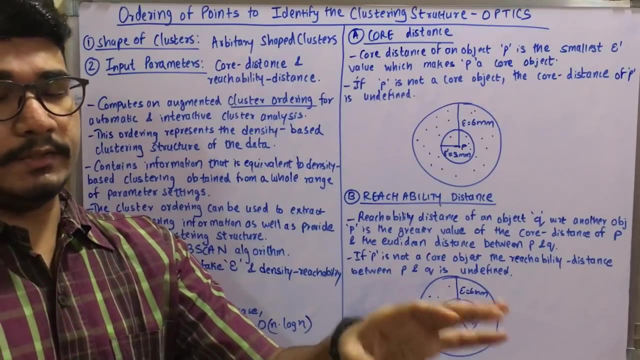 but it's the same for the quadratic time that we have. so we move on to the core principle, that is, the core distance and the reachability distance. so core distance of an object, p like any random object, any like, for example, any n number of data points might be there in that particular set. so 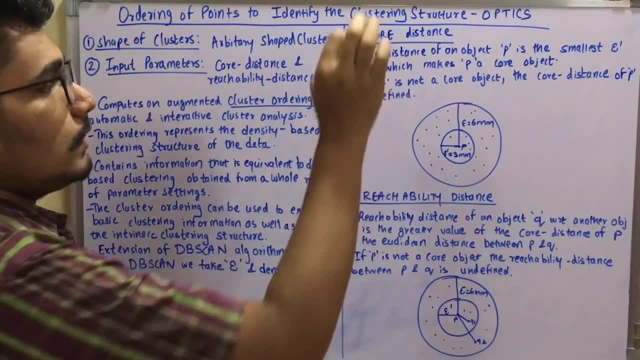 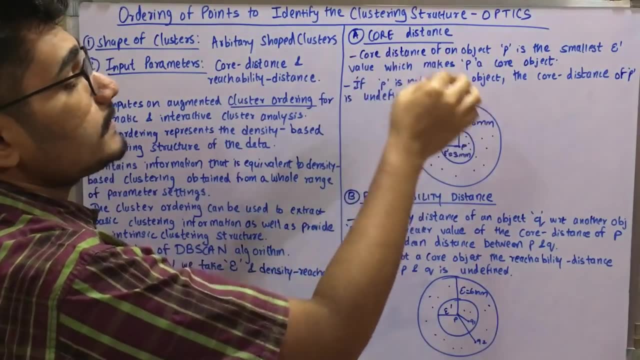 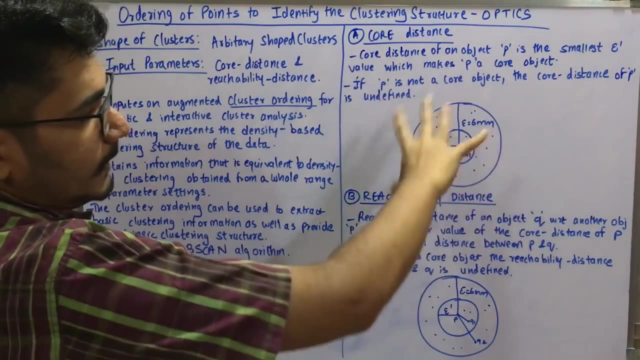 you will take any number of one particular random point so that if you assign as a core object, so core distance of an object, p is a smallest epsilon dash value which makes p as a core object, and if p is not a core object, then core distance of p is undivided. simple as that. and so we'll take this: 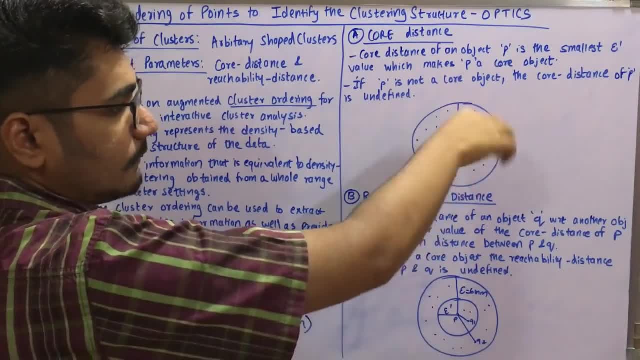 to concentric circles. so in this you have one inner circle and one outer circle. so the radius of inner circle is the radius of inner circle and the radius of inner circle is the radius of inner circle and the radius of inner circle is the radius of inner circle and the radius of inner circle. 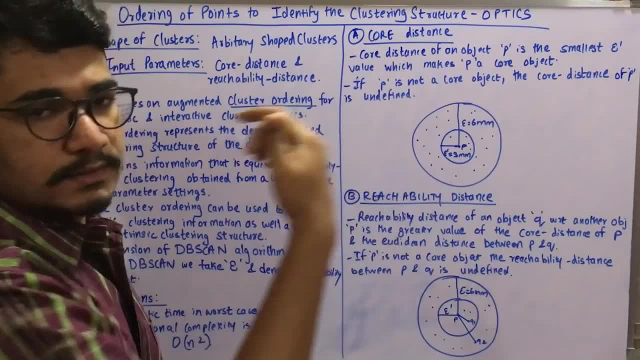 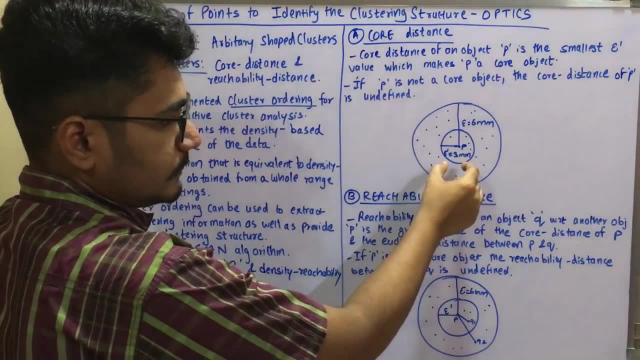 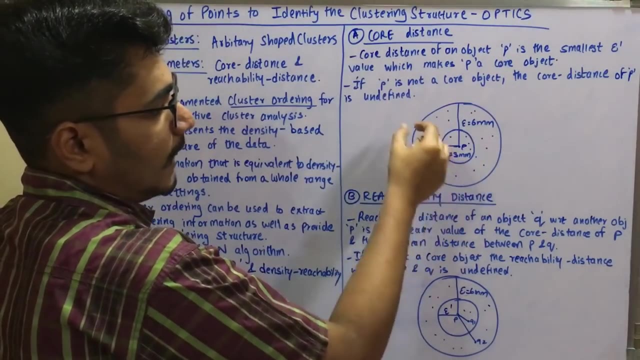 is 3 millimeter and the radius of outer circle is 6 millimeter, and so this, that is, this radius, that is this distance, is very small as compared to this one, and so since p's are core points, so core distance of p can be defined as epsilon dash, which is nothing but 3 millimeter. so, whatever i have, 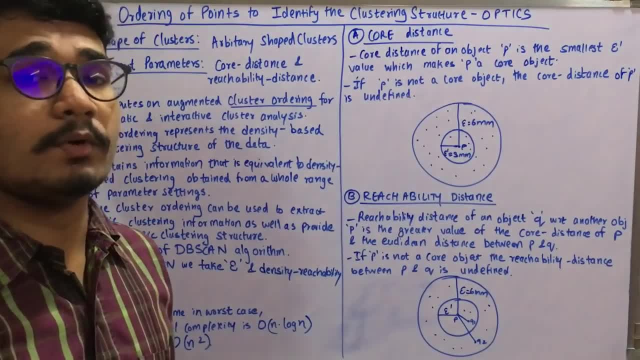 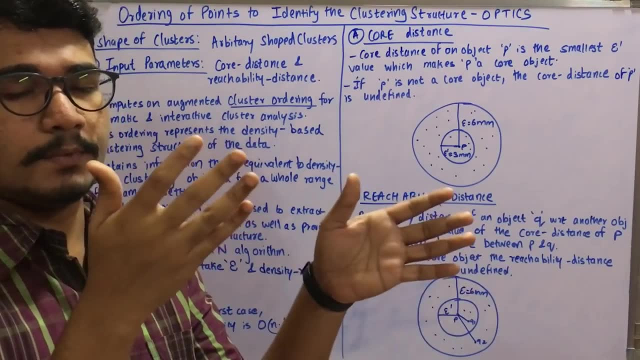 written is nothing but this thing. so the smallest distance we consider as the core distance, and when we move to reachability distance, it is nothing but it's. you compare two different objects, like from one distance you have to reach to another uh object, so like if you. 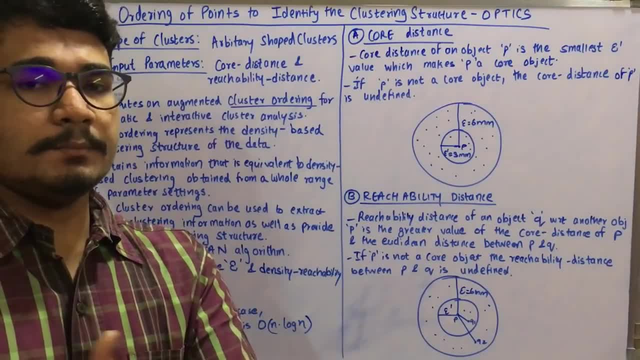 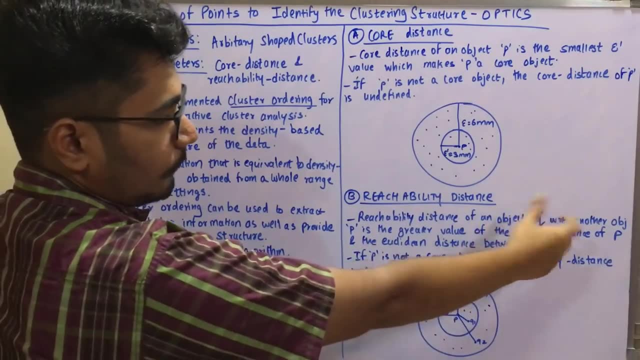 have q object and then you have to reach to p object. you need to have some reachability distance or how time or how long it will take to reach to that particular point. so it's between two points of an object q with respect to another object, p. it's a greater value of the core distance of p. 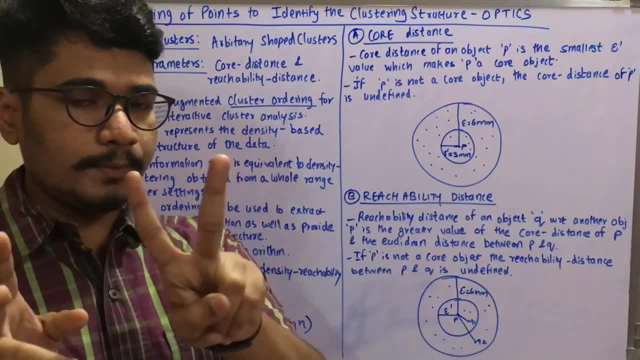 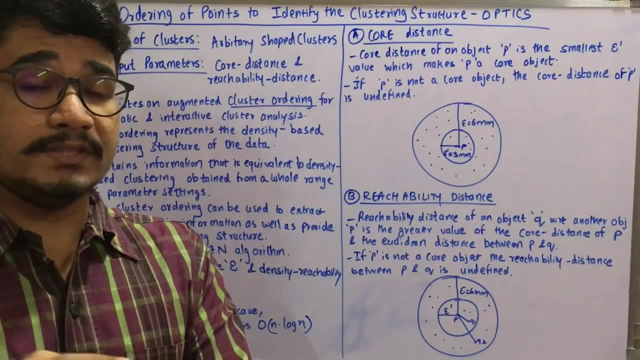 and the euclidean distance between p and q. it's like you compare or you take two parameters- that is core distance as well as the euclidean distance between p and q, and you can compare which is the greater value from that and then you assign that value is the reachability distance. 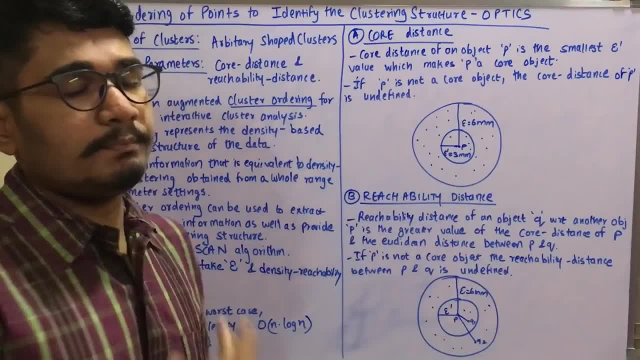 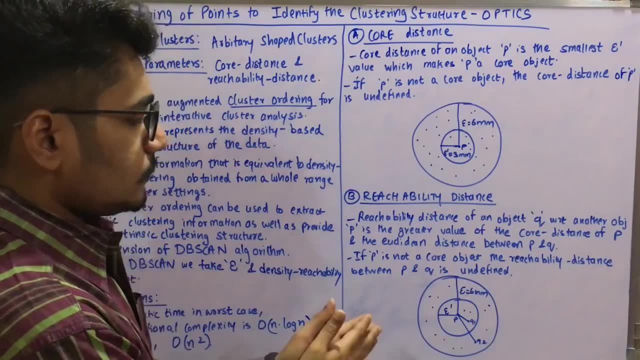 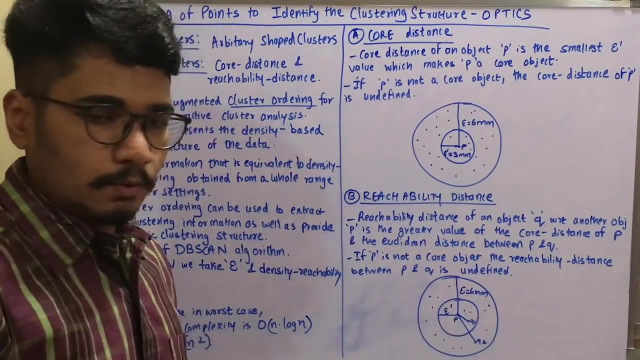 between two points, p and q, and, if so, in that also, if p is not a core object, then core uh is not defined and it's like: given an undefined value and so uh, you have this example like. similarly, you have two concentric circles, like i have seen, uh in this, and then you have the p as the core. 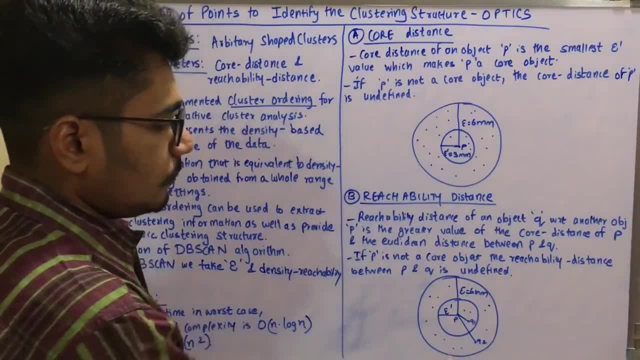 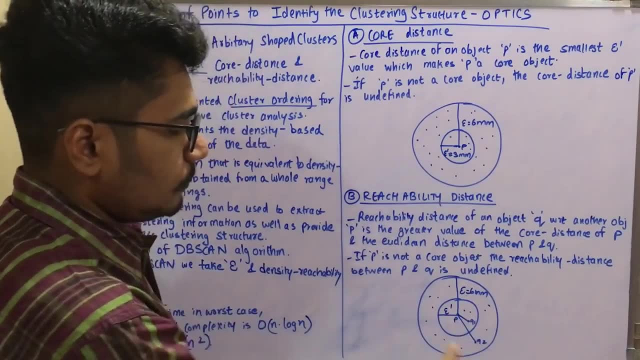 object and then you have two data points, that is q1 and q2, and so this distance is very small. so you can consider, as the radius, that is three millimeter and the outside one, that is q2, has six millimeters, so it's like the greater distance like, uh, this is the core distance and this is the. 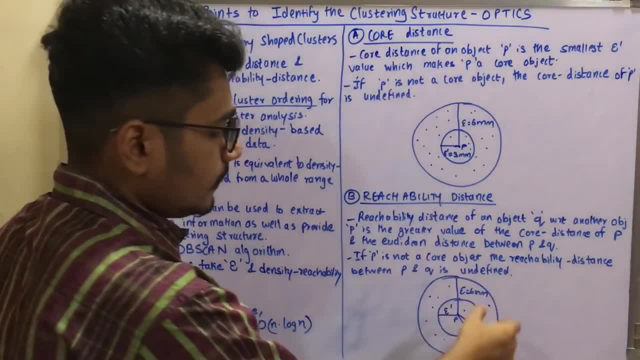 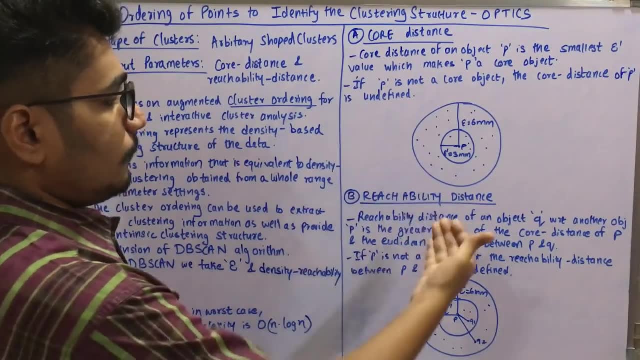 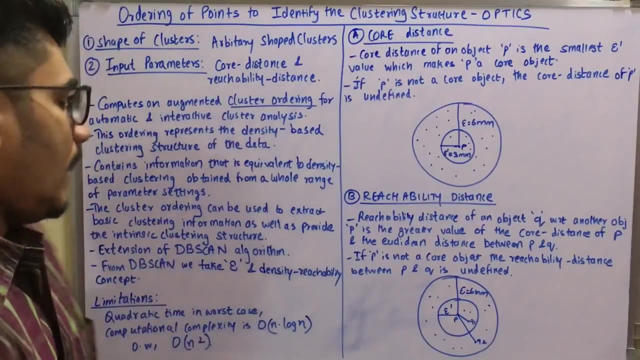 reachability distance, and so, uh, our outer radius, or outer distance of the circle, that is, having uh epsilon as six millimeter, would be considered as the reachability distance for uh, this kind of optics. so optics just revolves around these two concepts, that is, core distance and reachable distance. that's it. it's very easy, and the limitation is like, uh, similar for dps. can. 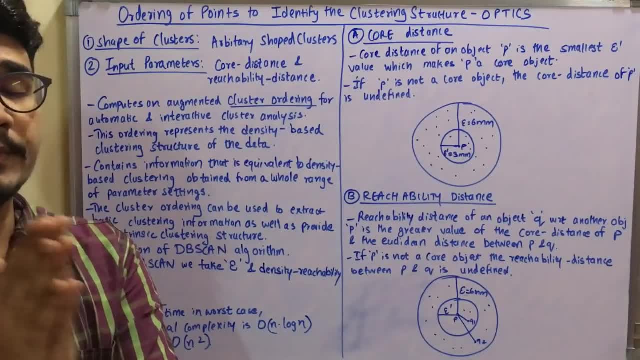 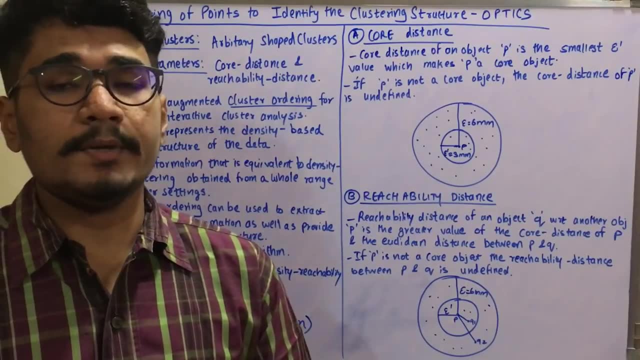 have the quadratic time that is in the worst case. uh, it has uh b go of n square and the normal computational complexity of b go of n log n. so well, that was all about regarding the optics technique in data mining, so hope you guys enjoyed this video from you. got educated by watching this. 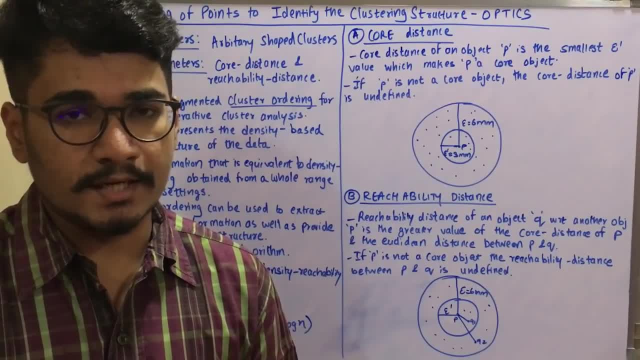 video. please do like, share, comment and, most importantly, don't forget to subscribe to my channel. thank you very much.